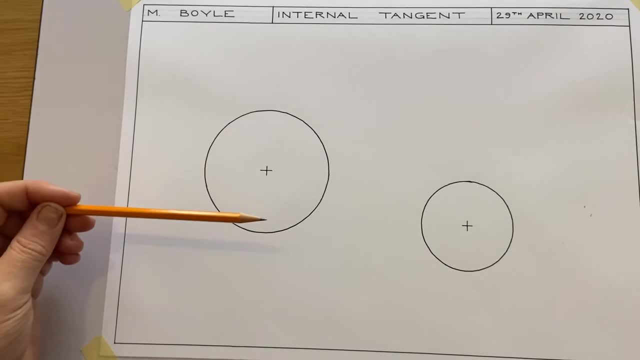 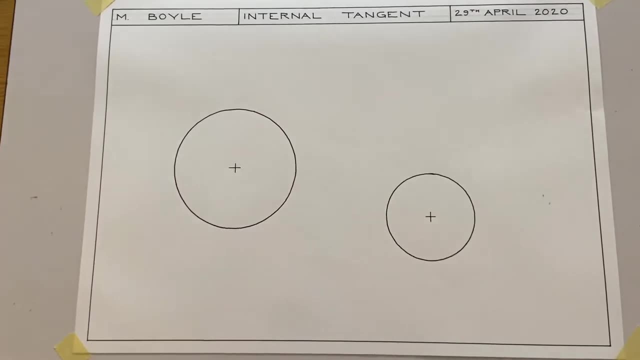 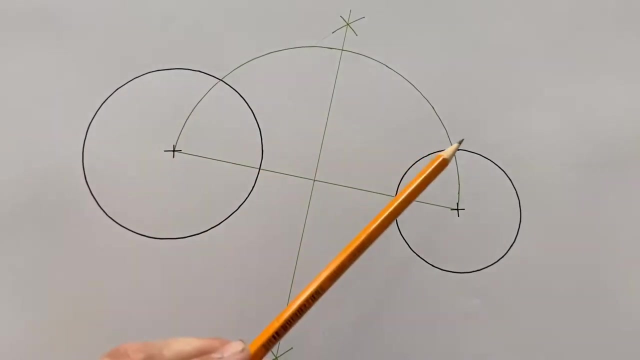 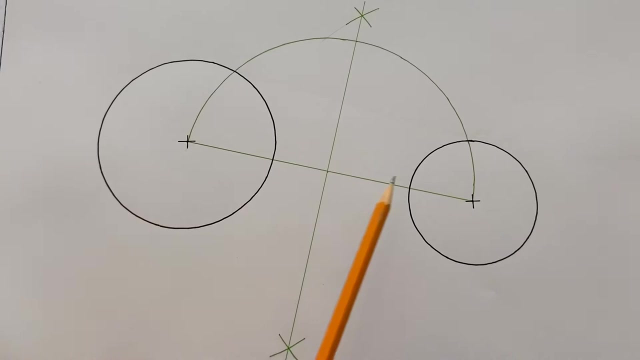 Radius 50, draw the large circle Down 40, across 160. and radius 35, draw the small circle on A3 paper. So, as with the external tangent, the initial construction for an internal tangent between two unequal circles is again to connect the centres together. bisect that line by taking a distance greater than half the line. 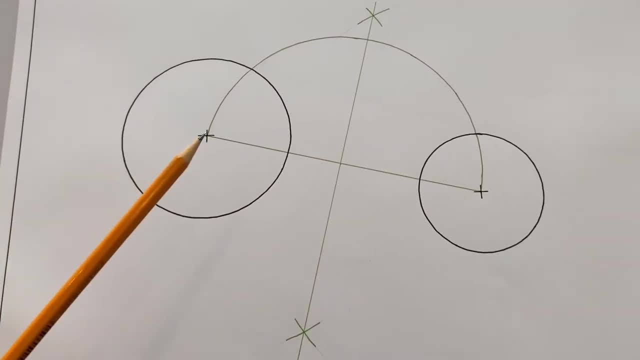 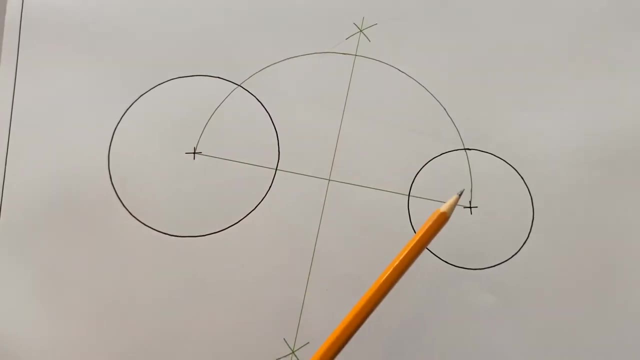 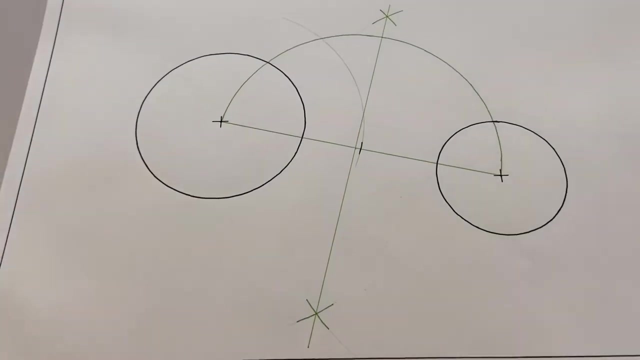 and swinging an arc above and below and then reversing your compass from this side, doing the same thing and drawing the bisector, and then draw a semicircle that will pass through both centres of the circles In the last construction, drawing an external tangent between the two circles. 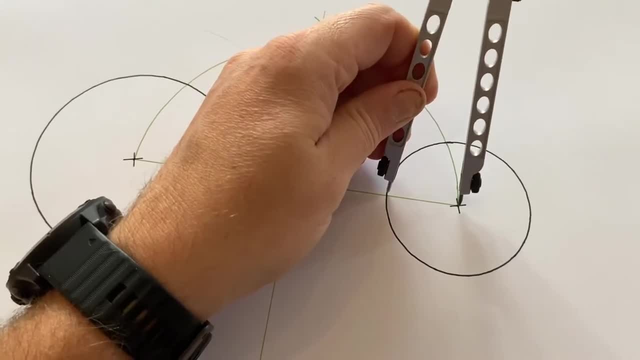 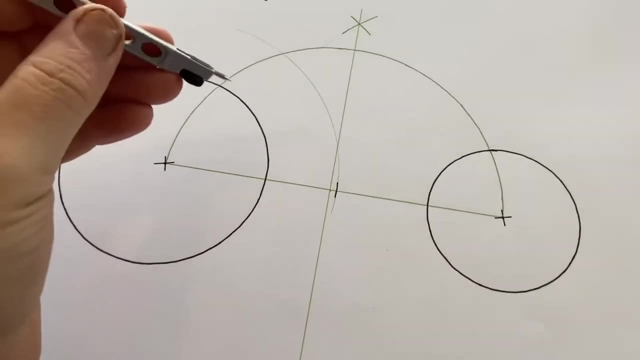 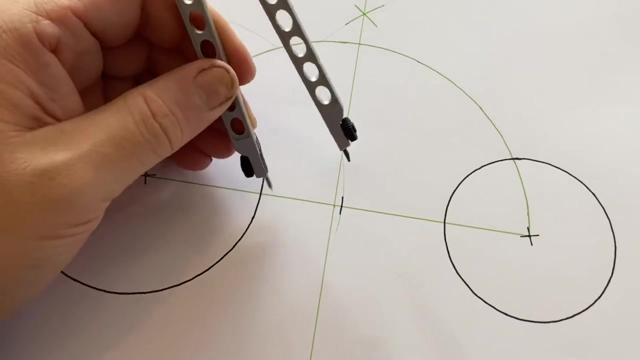 we took the radius of the smaller circle and then we subtracted that radius from the large circle. But to get an internal tangent between the two circles we now have to add the radius of the small circle. So, taking the radius of the small circle, we now have to add the radius of the large circle. 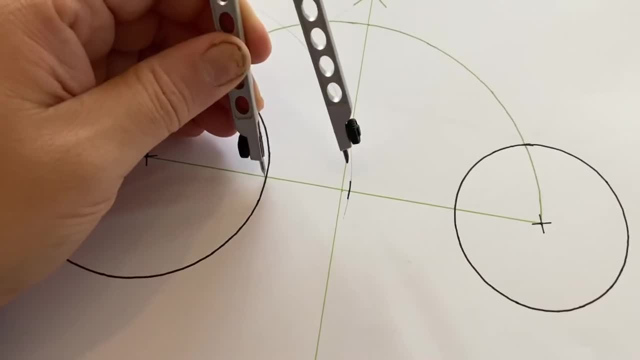 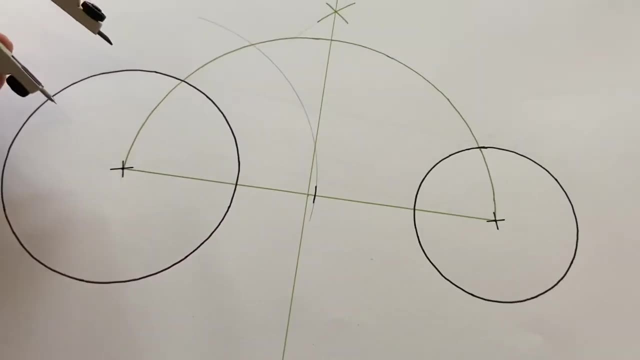 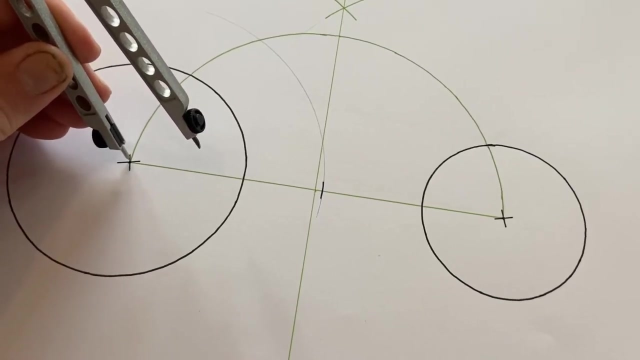 So, taking the radius of the small circle on your compass, placing it on the circumference of the large circle, and swing an arc, we add the radius of the small circle to the large circle. Then you place the point of your compass on the centre of the large circle. 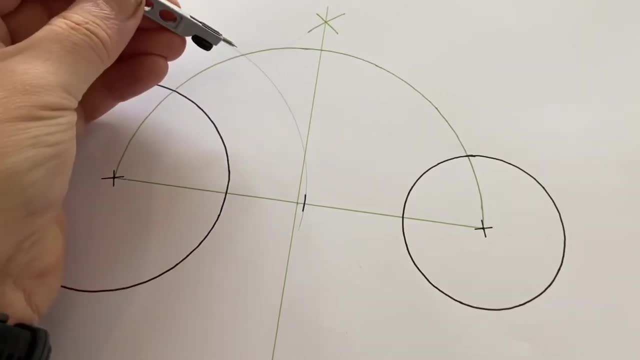 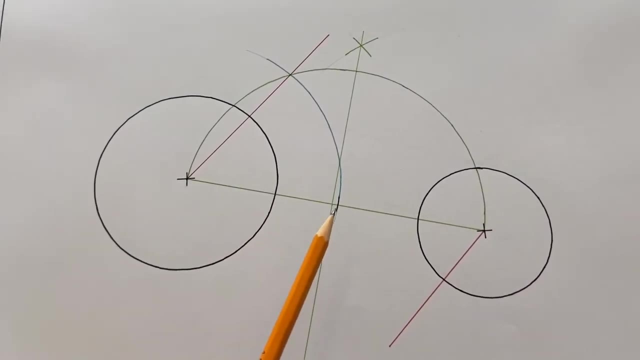 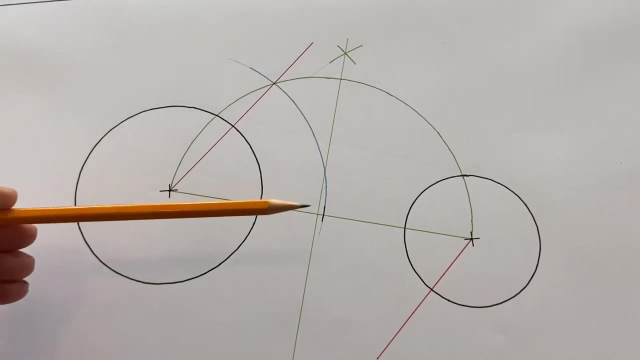 and you swing that distance up until it intersects the semicircle. So once we've added the radius of the small circle, we now have to add the radius of the large circle to the radius of the large circle. We place the point of our compass here. we open up the compass to pick up this point. 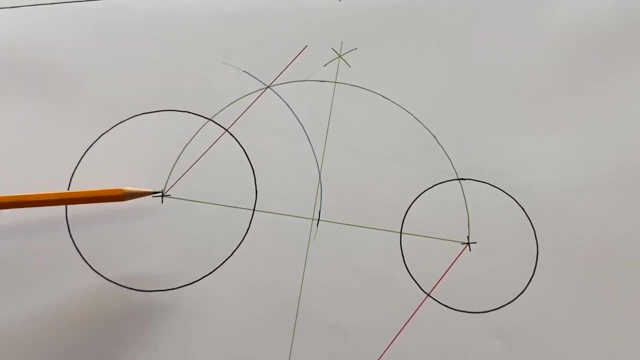 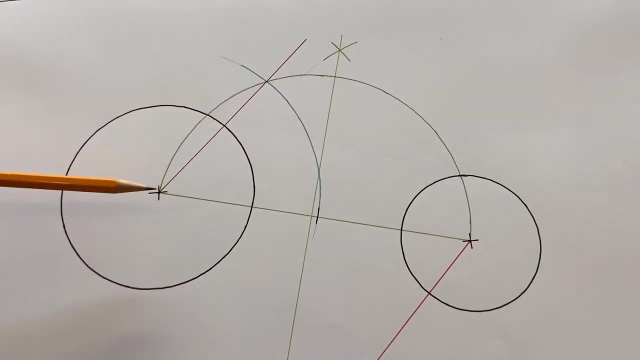 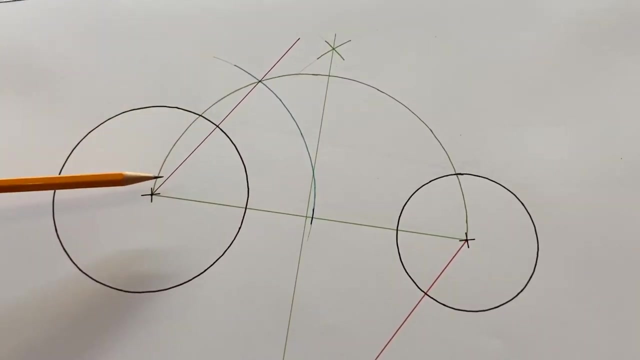 and then we swing an arc around the centre of the large circle. Where this arc intersects the semicircle, we draw the normal from the centre of the large circle through that point and that gives us our normal. Now, that will locate the point of contact, where the tangent 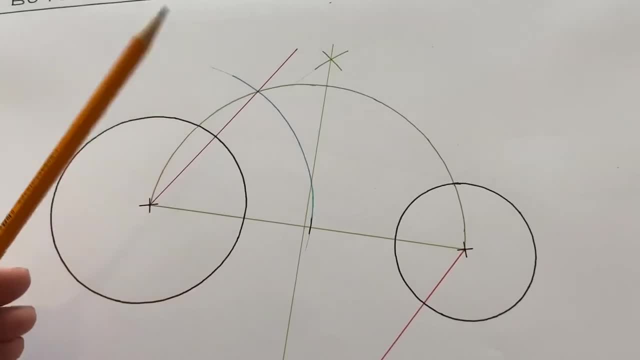 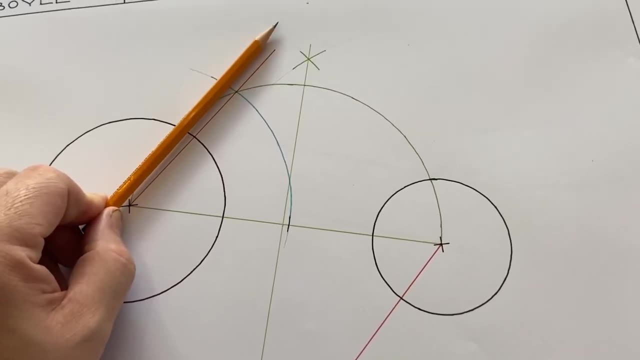 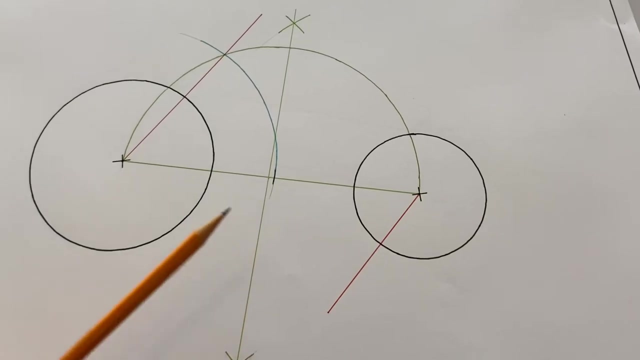 will intersect the circle here, then lining up our set square with that normal there and using sliding set squares we transfer that line down here and we draw the normal coming out in this direction here. So the normal up here is coming out on this side, but the normal on the 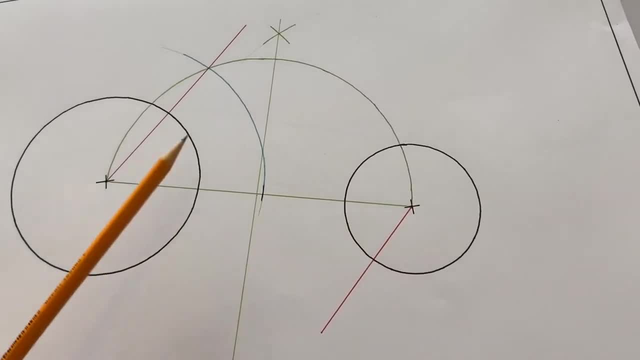 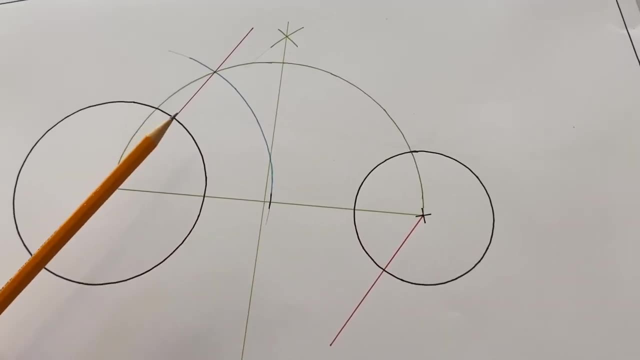 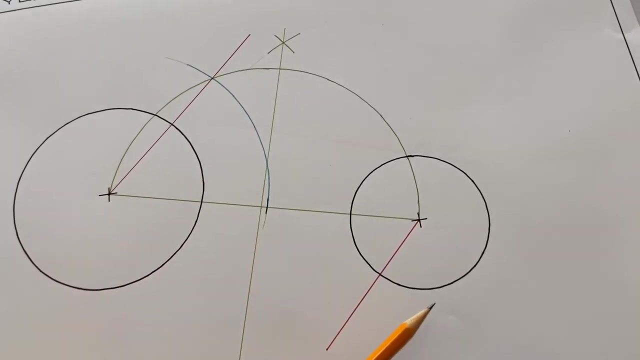 other side from the small circle has to come out through here in order to get the tangent in the position that we want it. So once we have the two normals drawn, we have the point of contact here, we have the point of contact here. line your set, square up with those and draw the tangent between them. 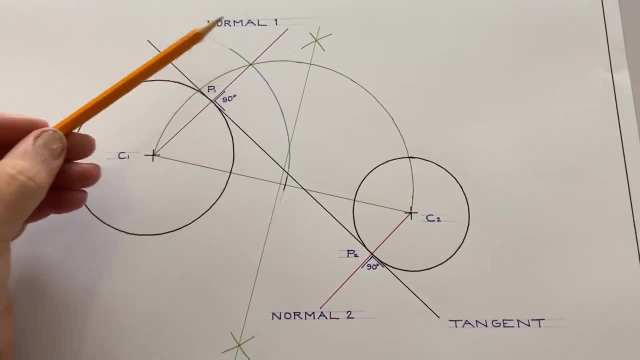 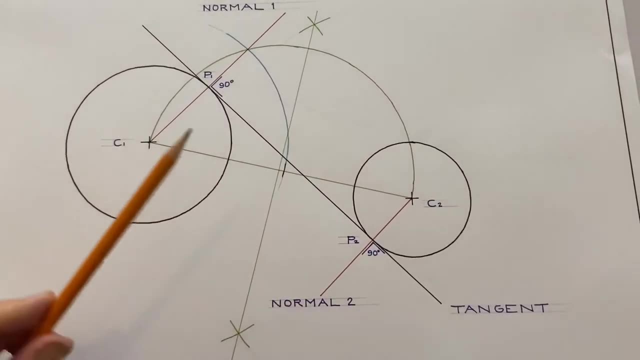 So when you draw your normal through here and you get the normal in this position and then, using sliding set squares, we draw the second normal coming out in the opposite direction. that will locate the point of contact on the large circle and the point of contact on the. 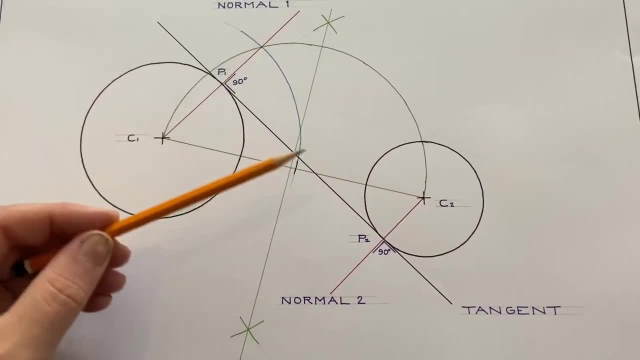 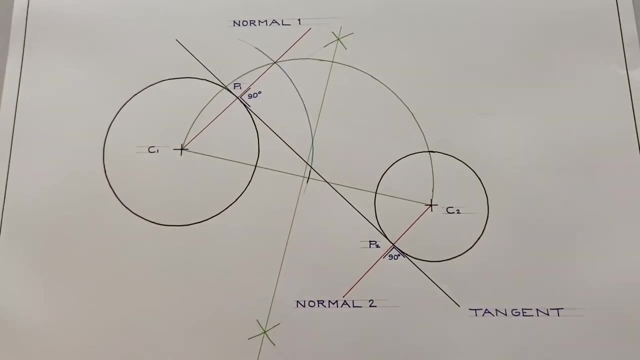 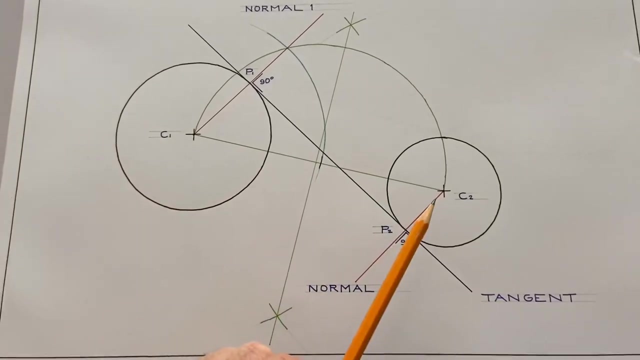 the small circle. and then we draw our internal tangent between the two circles in this direction here, So that there is the construction of an internal tangent between two circles of unequal radius. So connect the centers together, bisect that line, draw the semicircle, which is standard. 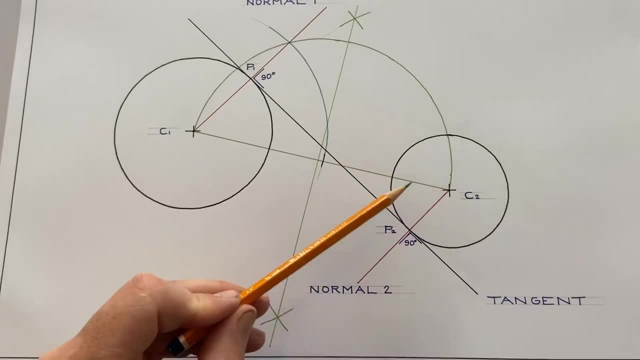 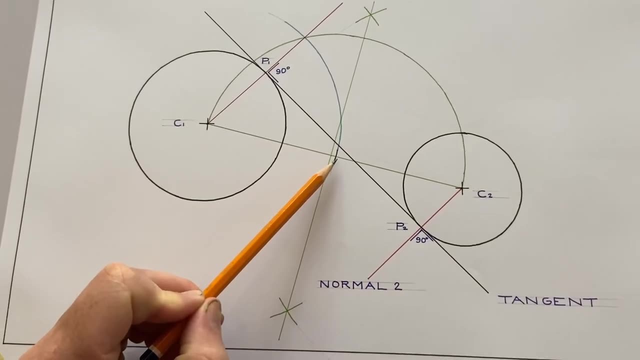 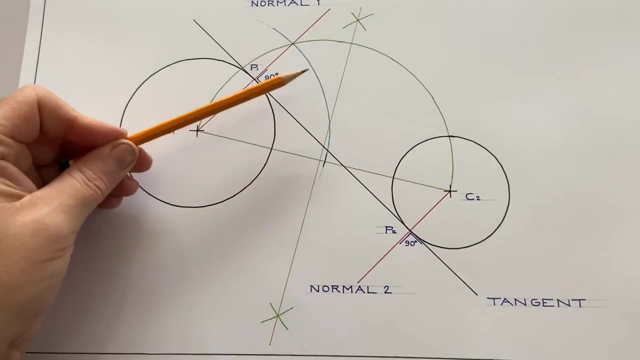 for all tangent constructions. Then you take the radius of the small circle and this time add it to the radius of the large circle Point of the compass on the center of the large circle and open it up to this distance and swing that up until it intersects the semicircle. 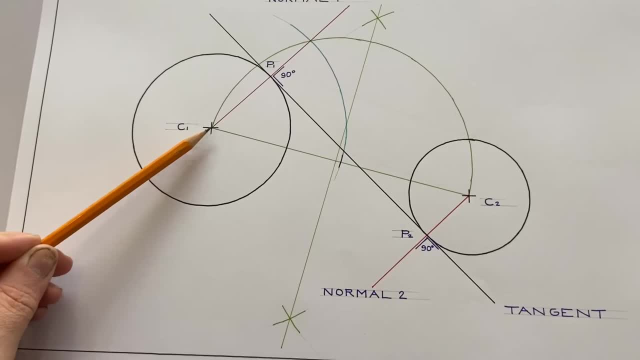 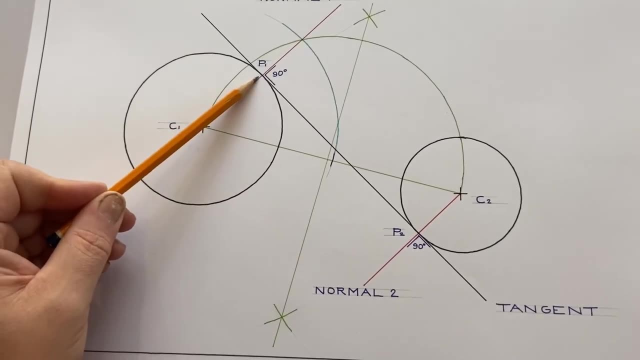 Draw your normal from the center of the large circle through that point where the arc intersects the semicircle, and that will be the center of the large circle. So that's the standard for all tangent constructions. Locate the point of contact on the large circle. Then, using sliding set squares, transfer that line. 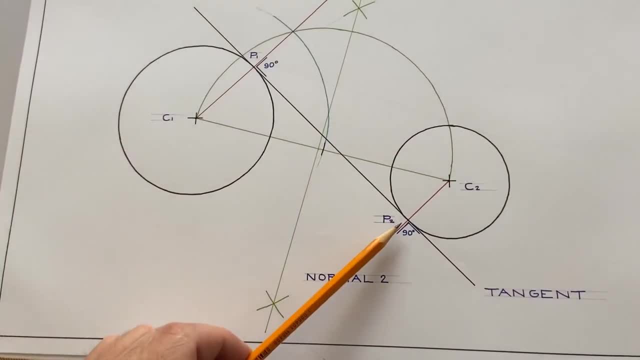 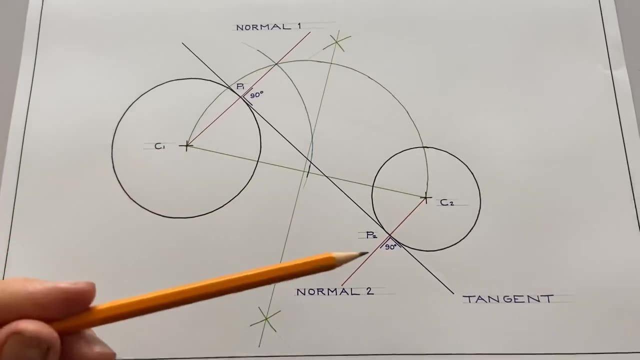 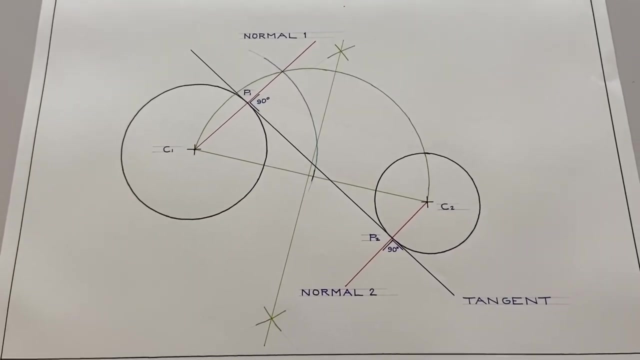 down to here and that will give you the point of contact on the small circle and then draw the tangent between those Again. label all important features: Tangent, normal point of contact on the circles. So that completes the drawing. Again put on the